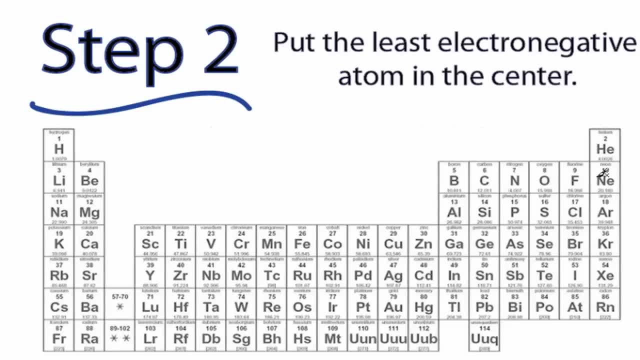 So how do you know? it's the least electronegative atom. Just remember that fluorine is the most electronegative, followed by oxygen. So as you move away from fluorine and oxygen, atoms become less electronegative. 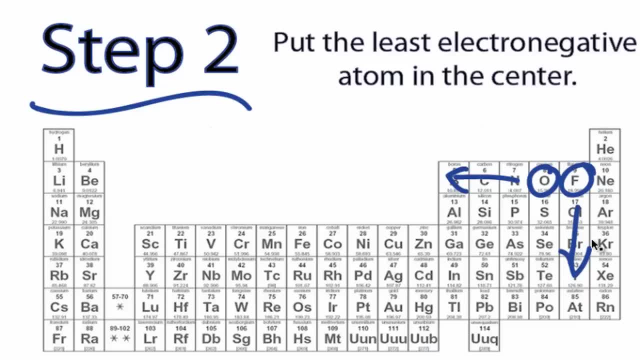 That means those atoms will go at the center. Let's see how it works. When I draw the Lewis structure for something like NO2, I can see that nitrogen is further away from fluorine than oxygen. That means when I draw my Lewis structure I'll put nitrogen at the center. 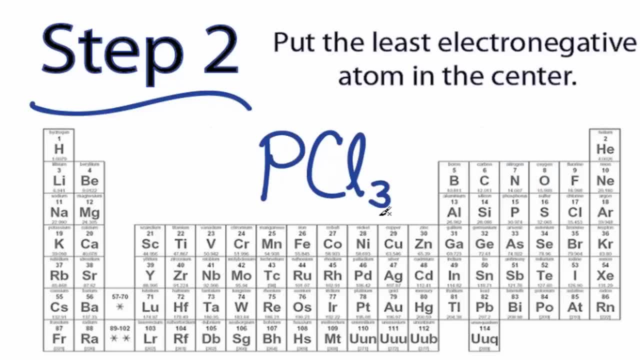 And oxygen's on the outside. For something like PCl3,, I can see that phosphorus is further away from the fluorine than the chlorine atom. So I'll put phosphorus at the center and the chlorine's on the outside, like this: 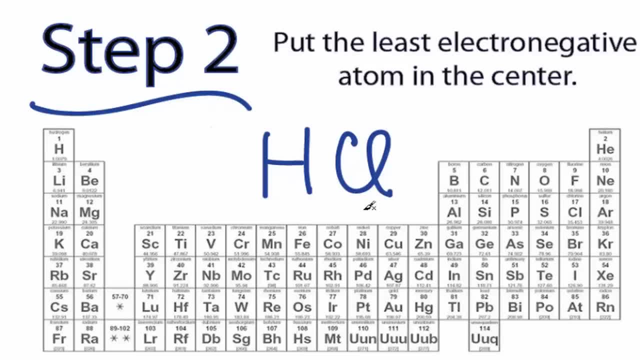 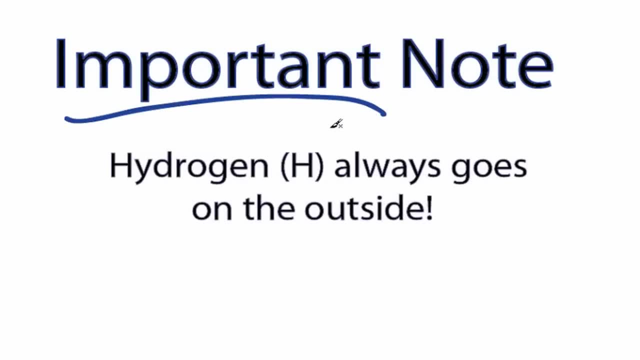 Some Lewis structures, like HCl, only have two atoms. In that case you don't have to worry about it, because there's no center. An important note: Hydrogen always goes on the outside of Lewis structures, Always, Seriously. 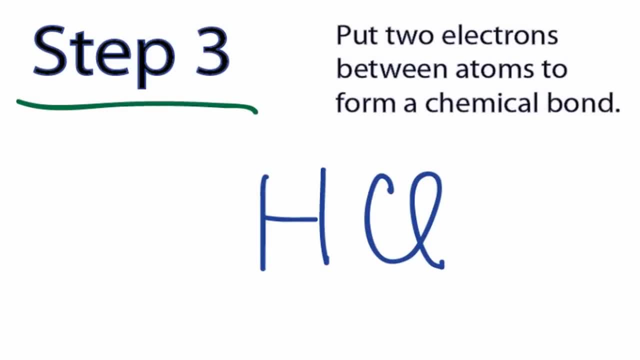 Let's look at HCl again. We know it has eight valence electrons and we'll put the first two in our structure between the H and Cl to form a chemical bond. That's important. By putting those two electrons there, we're showing that the hydrogen and the chlorine 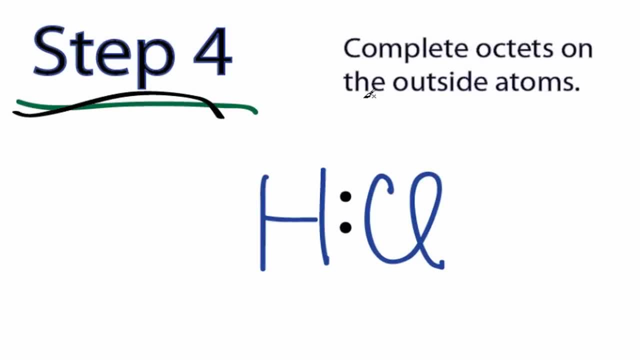 are chemically bonded. now Step four: Complete the octets on the outside atoms. Octet means eight For HCl There's a total of eight valence electrons, One for the hydrogen, seven for the chlorine. So we've used two already to form the chemical bond. 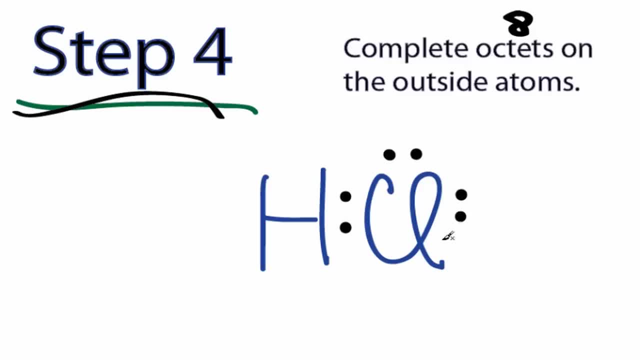 For the chlorine we'll put four, six and then eight. We've used all the valence electrons and we've completed the octet for chlorine. It has eight valence electrons For basic Lewis structures. the big exception is going to be hydrogen. 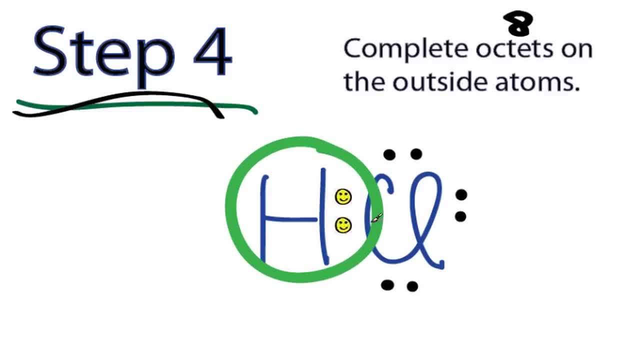 It only needs two valence electrons for a full outer shell, So hydrogen has a full outer shell. The hydrogen has a full outer shell with two valence electrons. The chlorine: its octet is full with eight and we've used only the eight valence electrons. 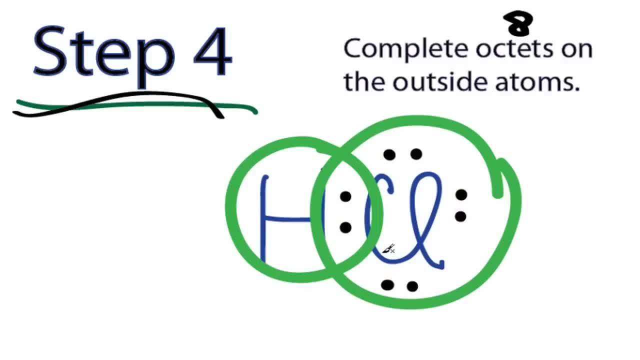 that we have for the HCl molecule. We're done with this structure. There's one more rule that we need to look at. It doesn't apply to HCl, and actually it doesn't apply to a lot of molecules, But what happens when you've used all your valence electrons and you still haven't completed? 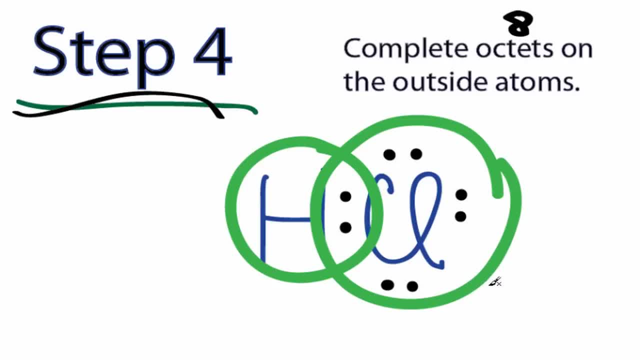 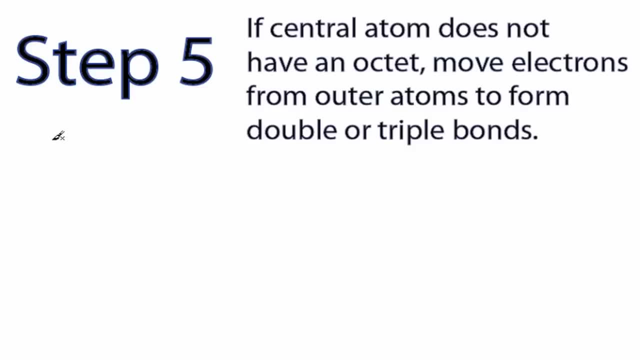 the octets for each atom in the molecule. That's step five. So sometimes you run out of valence electrons and still haven't filled the octets. Hey, it happens right. So in step five what we're going to do is, if we run out of valence electrons, we'll 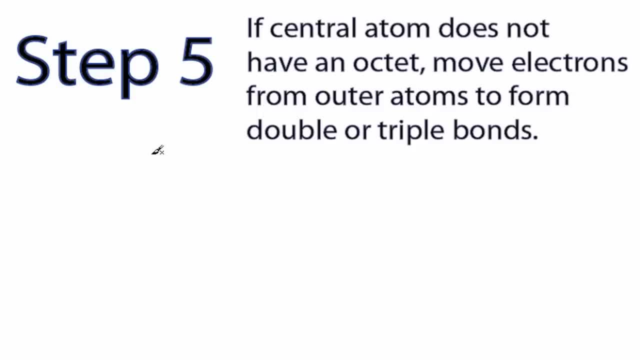 move some of the valence electrons from the outside to the inside and share them and form double and triple bonds. Here's how it works. So for O2, oxygen, if I follow all the rules, I count the valence electrons, I have 12,. 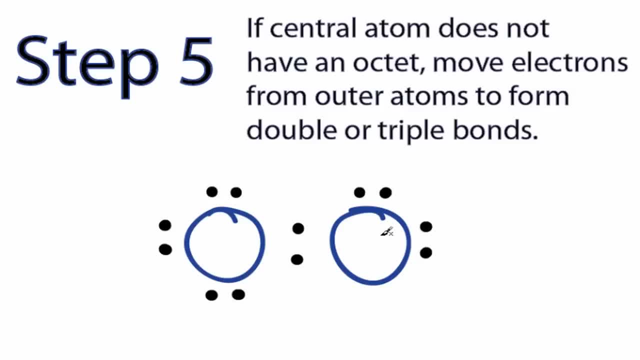 and if I put a bond between the atoms, I have 12.. So I have 12 electrons, I have 12 electrons, I have 12 electrons. When I move these two oxygen atoms and then fill the outer shell, I end up with the situation. 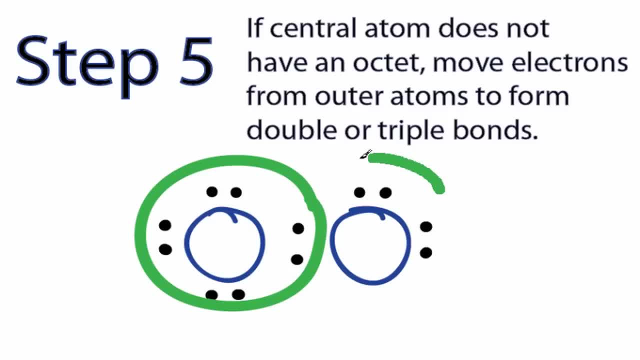 where I have an octet for this oxygen. It has eight, but this oxygen only has six valence electrons. It doesn't have an octet and I don't have any more valence electrons. To solve the problem, I can take these valence electrons right here and move them to the 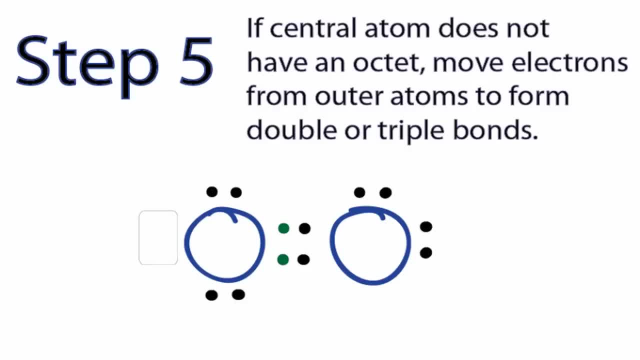 center to share them and form a double bond between the two oxygen atoms. I'm still only using 12 valence electrons, But now this oxygen has eight electrons. Now this oxygen has 2,, 4,, 6,, 8 valence electrons. and this oxygen has 2,, 4,, 6,, 8 valence electrons. 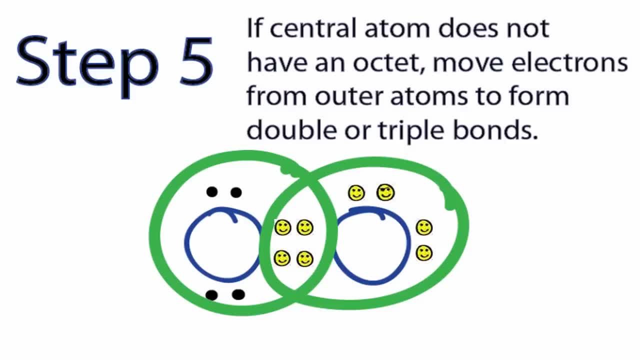 So by sharing those valence electrons I can get the octet on each of the oxygens and still use the 12 valence electrons that I had for the O2 molecule. If I wanted, I could replace these right here with two lines to show the double bond where. 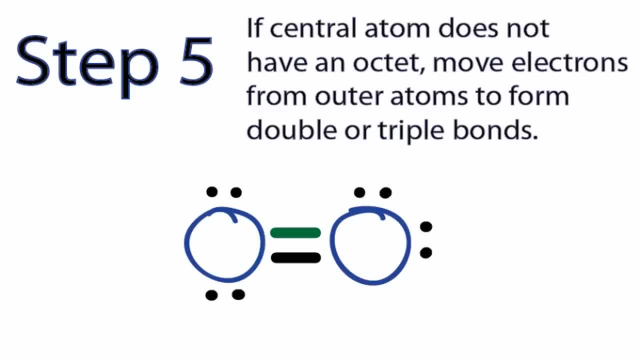 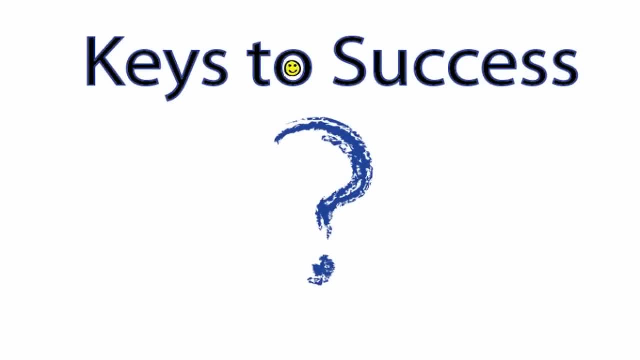 each line represents a pair of electrons. For Lewis structures like N2, I would even use a triple bond to achieve octets. So how do you get good at drawing Lewis structures? Well, the first thing is know the steps. They're your guide. 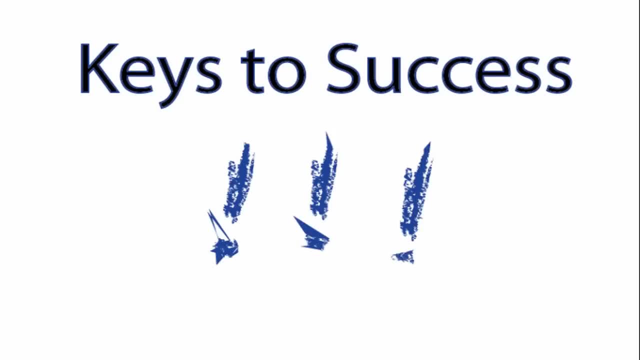 The second thing is practice. You need lots of practice to get good at this, for it to be second nature. Use the links in this video or go to my website and try more videos. First try it yourself and then watch the video. Pause when you're stuck. 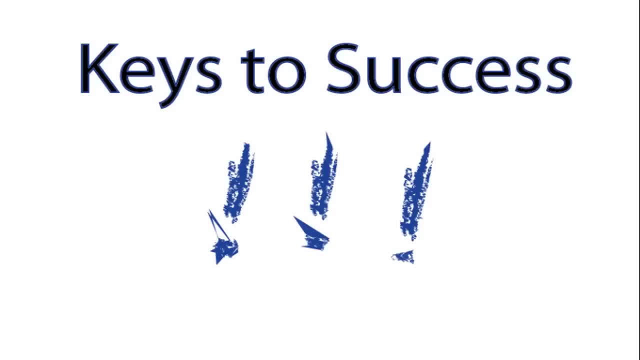 See what's going on And try to correct the problem. This is Dr B and thanks for watching.